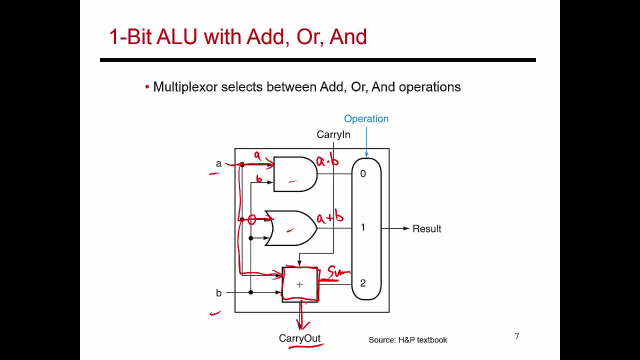 sent this way, okay, And the reason it's being sent down will be made clear shortly. You'll also see that there is a carry-in coming from here which is also being fed into this add unit, right? So potentially, this add unit is adding the values of A, B and a carry-in. 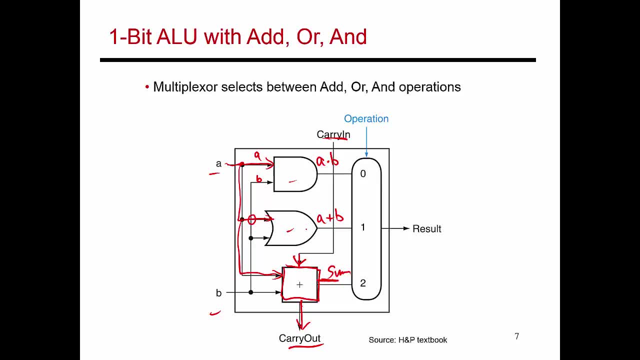 producing a bit for sum and a bit for carryout, For starters. you know, let's just assume that there is a carry-in. I won't go into details of where that carry-in is being produced from just yet. okay, But these are the three inputs: A, B and carry-in. Accordingly, the two input bits are: 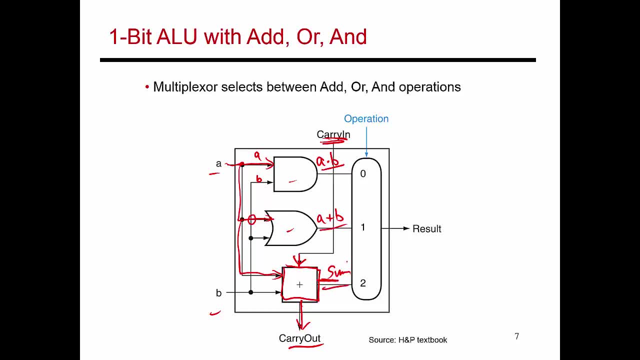 being ANDed or they're being added to the carry-in bit to produce a result. Now the output of this ALU is going to be only one of these three operations. okay, So I have a multiplexer over here Which is then going to connect one of these inputs to the output, And which input I connect? 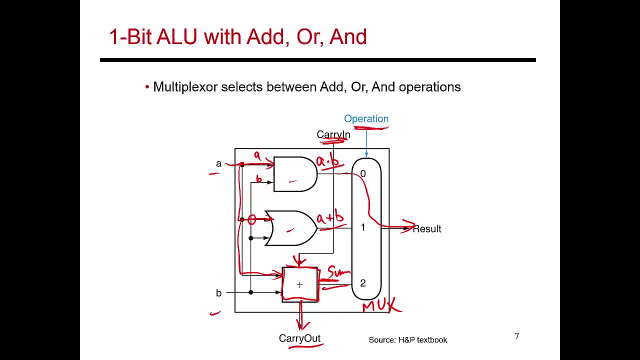 to the output depends on my operation code. So I have an operation code- let's say 00,, which says that I'm trying to do an AND operation. I have a code 01 that says I'm trying to do an OR operation And a code 10 that says I'm trying to do an addition, that is, I'm trying to add up. 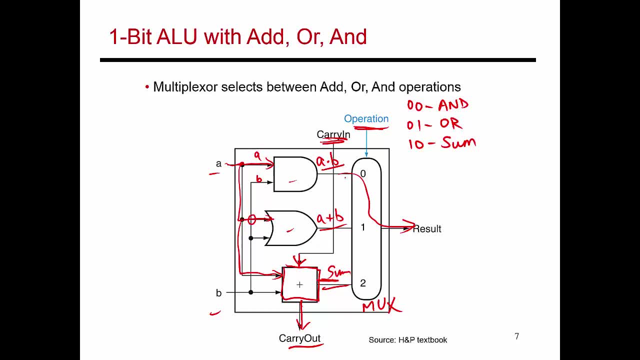 the two input numbers. So, depending on the value of this code, one of these inputs gets connected to the input. So in order to use this one-bit ALU, I have to provide two one-bit numbers as input And I have to provide an operation code telling what kind of operation I want performed on. 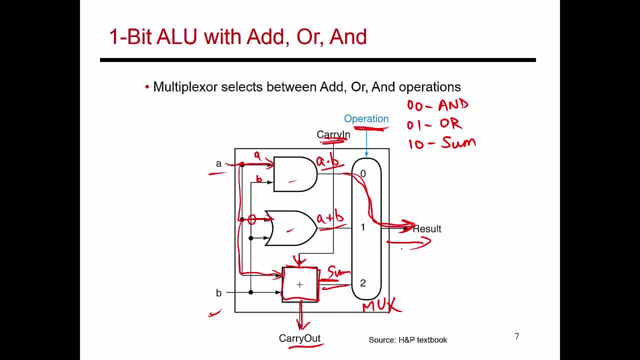 these two input numbers And that's the result that emerges from this black box. So you can see that this one-bit ALU is fairly easy to design with a few gates, right? So in previous slides we've seen that you know, you just need a handful of gates to implement. 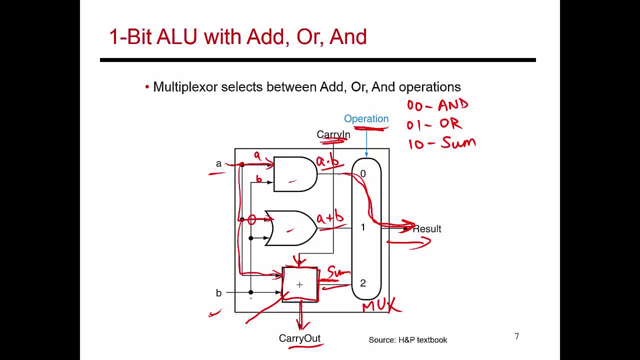 this adder right. So you're just going through two sequential gate delays to produce a result. Similarly, we saw a diagram for the multiplexer as well. Again, you're going through two sequential gate delays to produce the result. So this entire circuit is very simple and is capable. 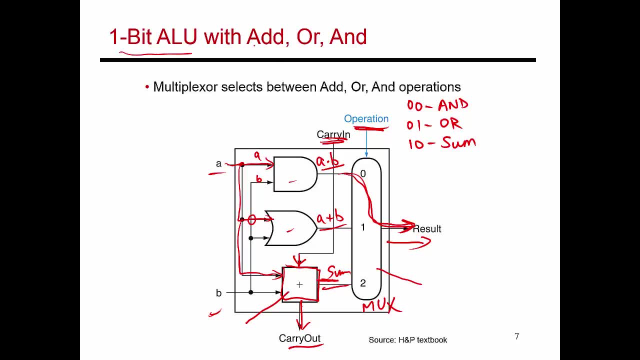 of this very simple operation where you're just adding one-bit numbers and performing these three operations. Now let's add more to this right. The first thing I'm going to add is make this ALU capable of handling more than just one bit right? So in our MIPS, 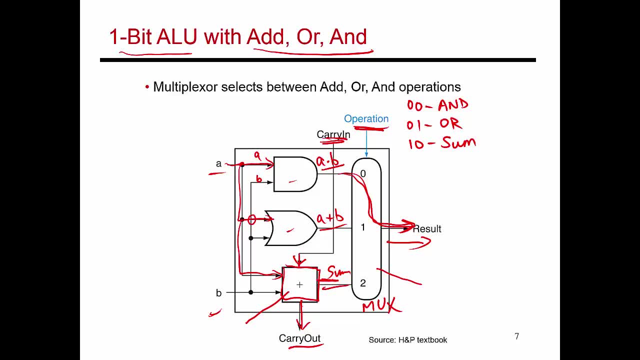 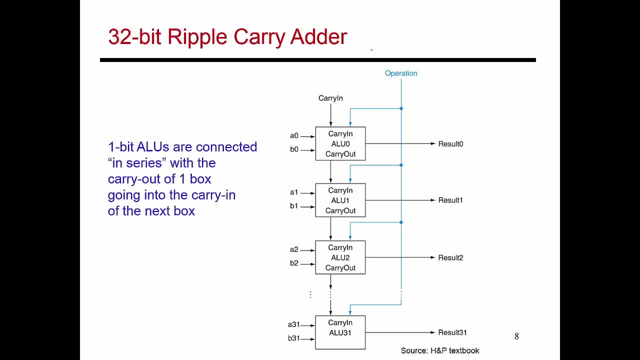 architecture. we were dealing with 32-bit values for the most part. So how do I do addition to 32 bits? So what I'm going to do is take this basic one-bit ALU and chain it together, right. So this box over here represents the ALU that I showed you on the previous slide. 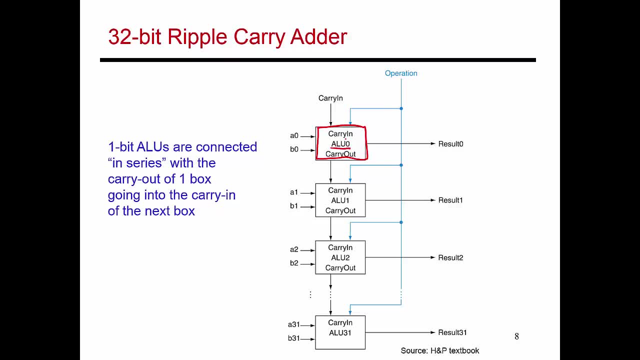 So this is referred to as ALU0 because it deals with bit numbers 0.. So if I'm giving a 32-bit value A and a 32-bit value B, the first bit of A- A0, and the first bit of B. 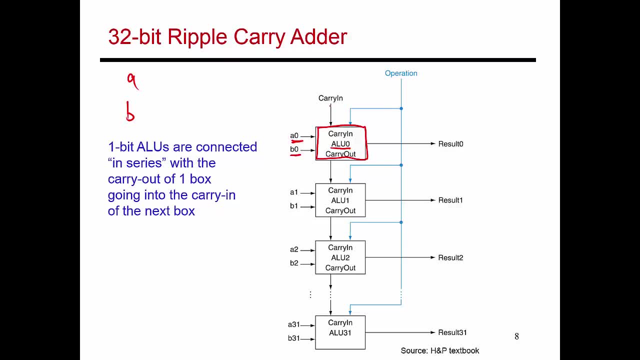 B0, are fed as inputs over here. In addition, I have a carry-in. Since these are the first bits, the carry-in is definitely going to be a 0 while I perform this addition. So let's say, I'm trying to do an addition, so the operation code is going to be 10, and so the result. 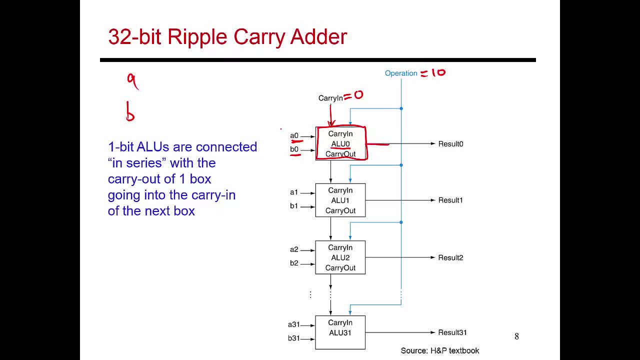 coming out of here is the sum of A0 and B0.. There's also a potential carry-out that is generated That feeds as input to the addition of the next set of bits. right, So there's ALU1 over here, which is going to deal with adding up bit number 1 of A bit number 1. 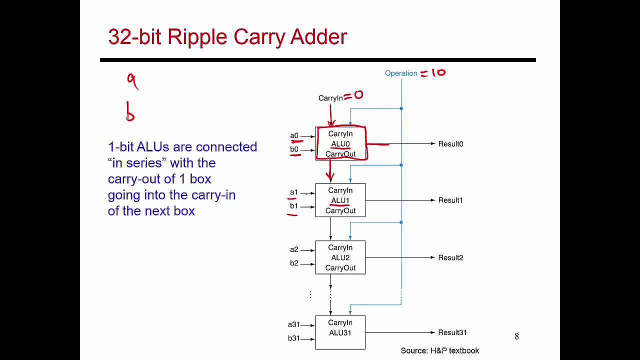 of B and any carry that was generated from the addition of bit number 0, right. So that's why I had the carry-out coming at the bottom, because the carries are basically fed to the next stages And the carry-in comes from the top right. So ALU2's carry-in is the carry. 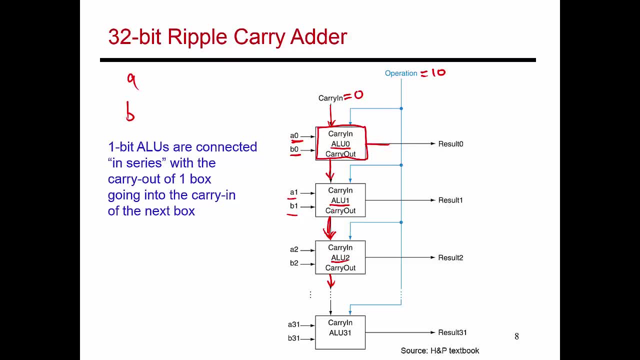 that was generated by ALU1.. So when I'm performing an add, I provide these 32-bit numbers as input, I feed a carry-in of 0, and the addition keeps happening, one ALU at a time And ultimately the 32nd ALU. 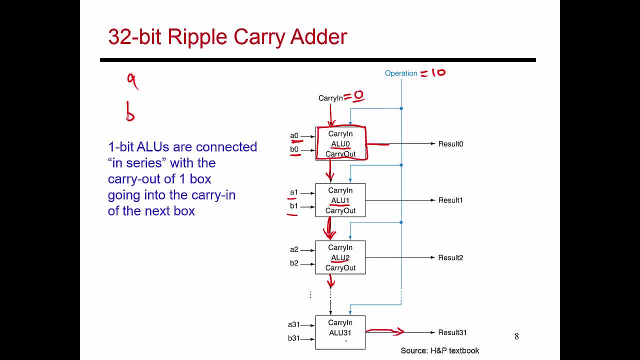 produces its final result, the final sum, right, And it also produces a carry-out, which I'm going to ignore for now- right, But that's potentially an overflow bit which I'm going to handle later. If, instead, I gave an operation code of 00, that means I'm trying to do an AND What I 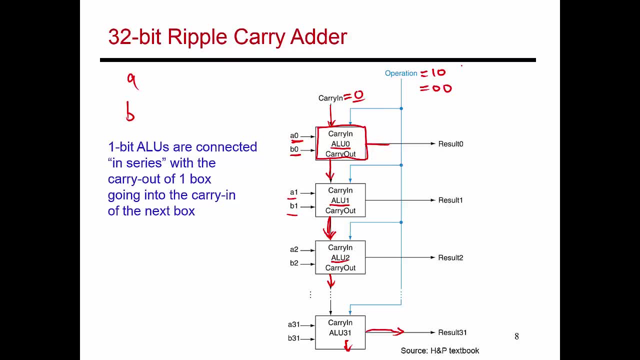 need to perform is a bitwise AND So each one of these ALU blocks is going to take its corresponding input. So ALU0 is going to take inputs A0, B0,. do a bitwise AND of those two bits And that's the result over here, And that'll be bit 0 of the result, And similarly ALU1,. 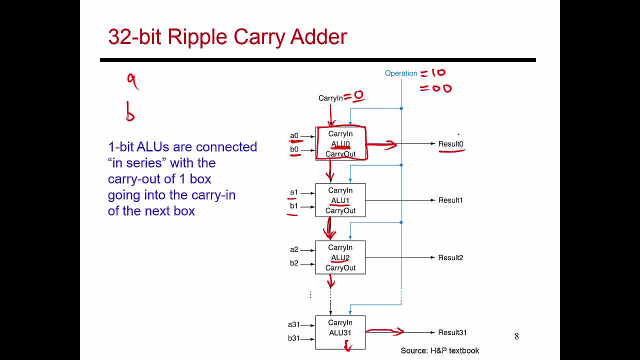 ALU2, they all do their independent AND operations, So there's really no carry-out or exchange of information between these different ALUs if you are performing an AND or an OR operation. So it's only the addition that, in this case, requires the carries to be propagated from. 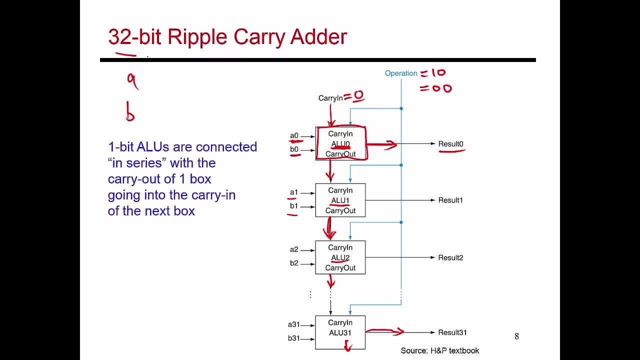 one ALU to the next. This is therefore referred to as a 32-bit ripple carry adder, because the carry is rippling from that. So that's the reason why the solution is so important. It's just because the operation is coming across enough times. theận operation, which 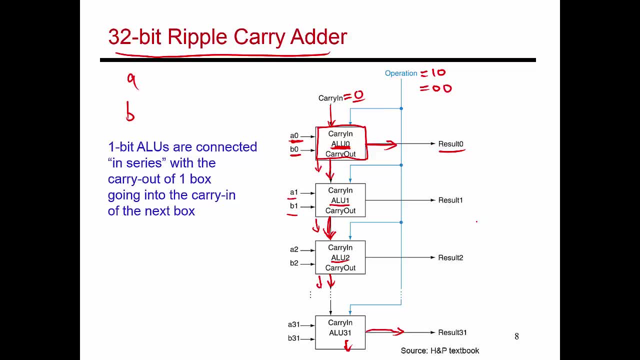 normally takes a little more time isbarrier than ALU0. And so this doesn't just involve a few additions, It also takes a little extra amount of time. So we said that going through one of these blocks over here requires close to a handful. 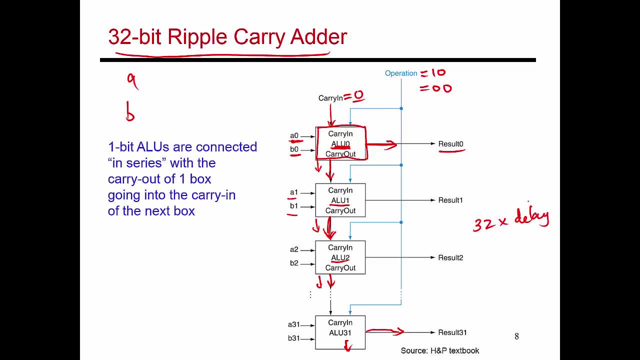 two times the delay for each of the one-bit ALUs, So this is going to be certainly more time consuming than the basic one-bit ALU that we had designed before. Now let's add a few more things to this basic ALU. Let's add subtraction. 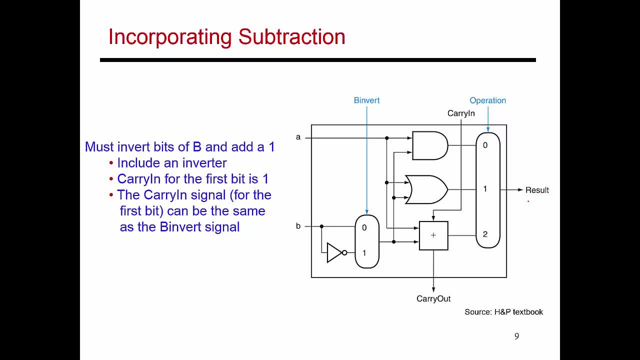 And it turns out that adding subtraction is not a huge change. So if you're giving me two input numbers, A and B, if I want to subtract and do an A minus B, the way to do it is: do A plus B, bar plus 1.. 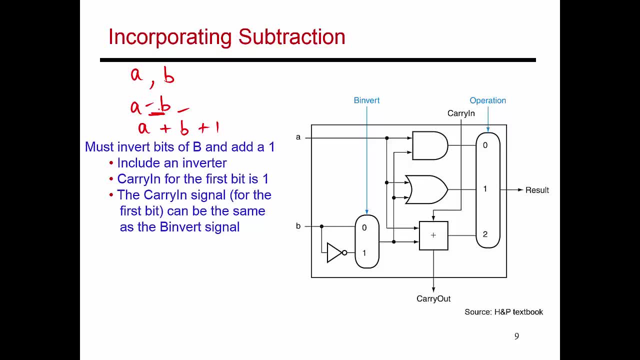 So adding minus B is the same as computing the two's complement of B, which is done by inverting the bits of B and adding a 1 to it. So if I'm giving you inputs A and B and I want a subtraction to be performed, what I essentially 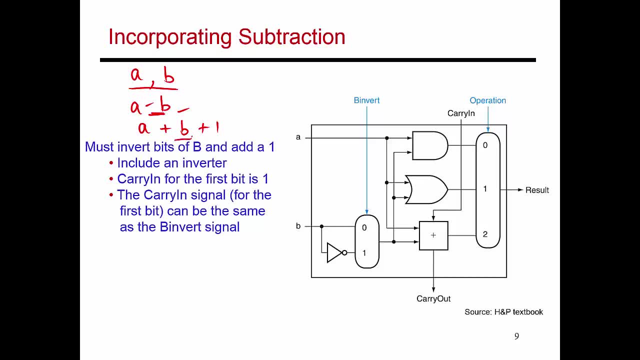 need to do is invert all the bits of B before performing the addition, And then at the very end I also need to add a 1 to it. So the way I do it is: as soon as B comes in, it also gets fed to this. 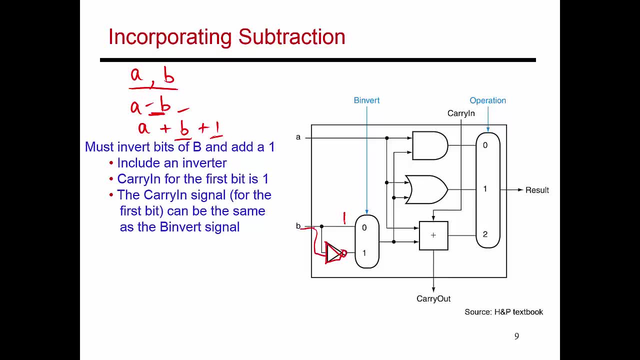 This inverter gate over here. So what comes in here is the value of B itself in its raw form. What comes out over here is the value of B inverted, so B bar, And then I'm going to use a multiplexer to decide what then propagates through the rest of the circuit. 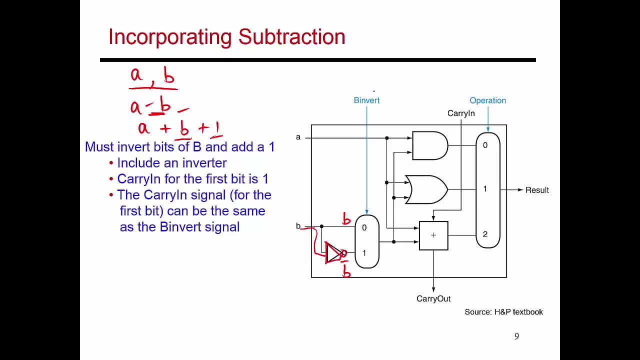 Should I be adding a B or should I be adding a B bar? So there's a B invert signal. If I assert that signal, then what comes out of this multiplexer is B bar. If B invert is set to 0, then what? 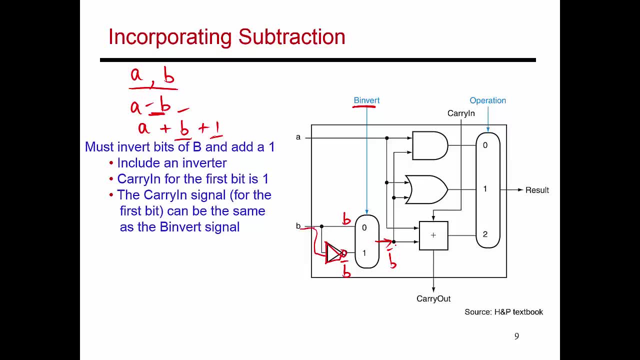 comes out of the multiplexer is the value of B itself. So if I'm trying to do a subtraction, I'm going to set this bit to 1, which means that what emerges from the mux is B bar, And then what enters this adder over here is A and B bar. 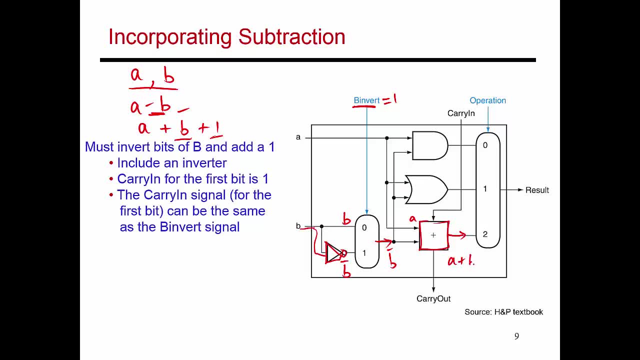 So what comes out of this adder over here is A plus B bar, So we are nearly done. There's still this 1 that I need to add, And the way I do that is: I go back to the circuit here And I see that when I'm doing addition. 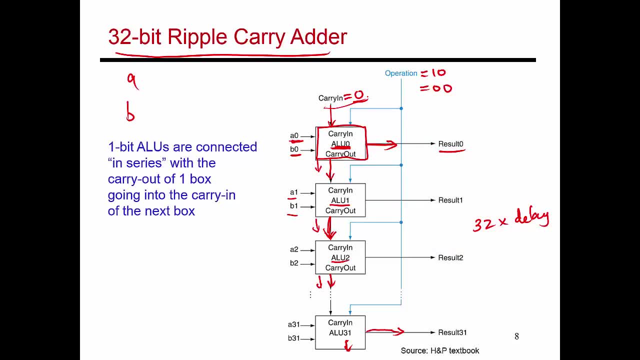 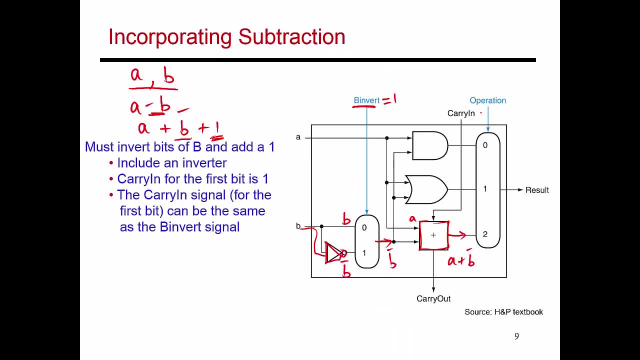 I set the carry in of 0.. If I set the carry in to be 1, then I'm going to add a 1 to the result. So if I'm doing a subtraction instead of setting the carry in to 0,. 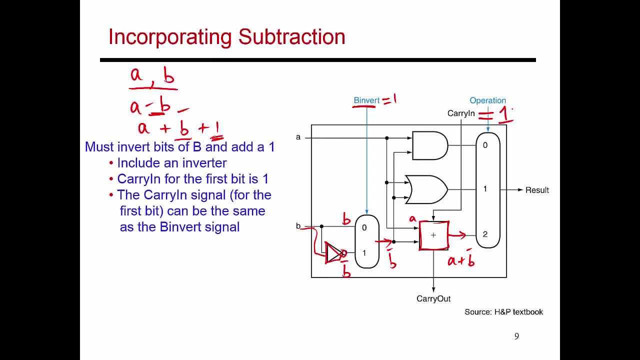 I set the carry in for the very first bit to be equal to 1.. And that automatically adds a 1 to the result. So what comes out of this adder is A plus B, bar plus 1.. So by adding these few additional gates, 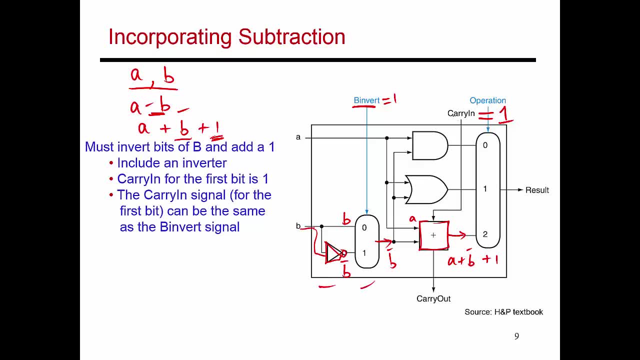 essentially an inverter and a multiplexer, and by being able to set this carry in sometimes to 0 and sometimes to 1, this 1-bit ALU is now capable of performing subtraction. Now note that this carry in of 1 is only. 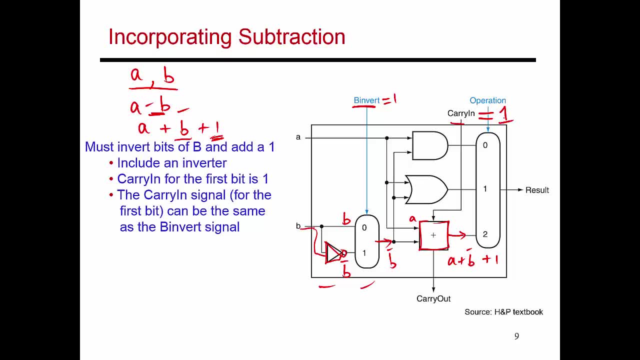 set for the very first bit. Once I've done that, if additional carries are being generated, those will get automatically propagated to the next few bits. I don't have to keep adding a 1 to each one of the individual ALUs. It's only the very first ALU that needs to add an extra 1.. 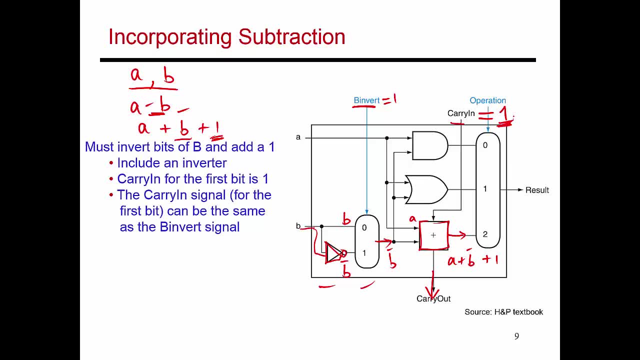 And that is achieved by just setting this carry in to be 1.. The rest of the circuit is going to behave exactly as before. So if I again look at the control bits, remember That 0, 0 indicated that I wanted to do an AND. 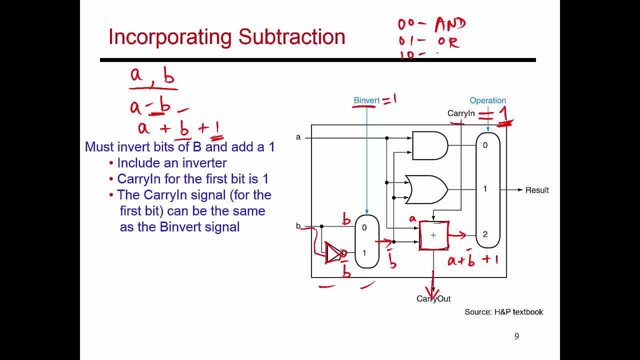 0, 1 indicates I want to do an OR. 1, 0 indicates that I want to do an ADD. If I want to do a subtraction, I'm still going to provide a code of 1, 0, because there are only three inputs to this multiplexer. 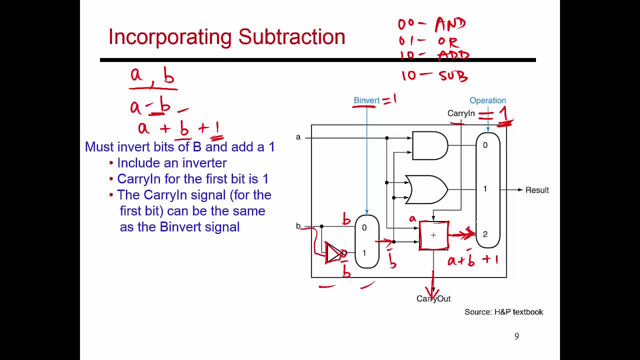 And I want to continue to use whatever is being produced by the adder. So, even for a subtraction, the operation code is going to be 1, 0.. But what I also need to do is that the B invert signal has to be set to 1, in this case. 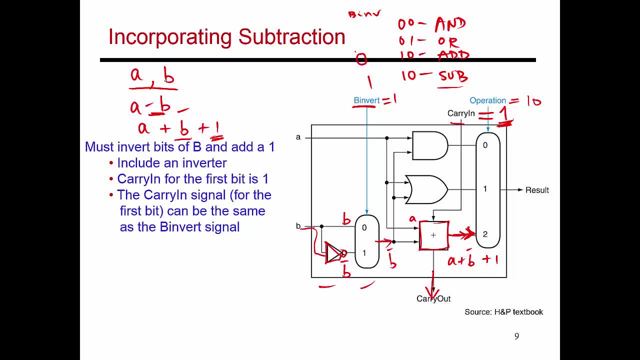 And in case of an addition, the B invert signal is going to be set to a 0.. In case of an OR and an AND, also the B invert signal will be set to a 0.. So I've introduced one more input signal, which 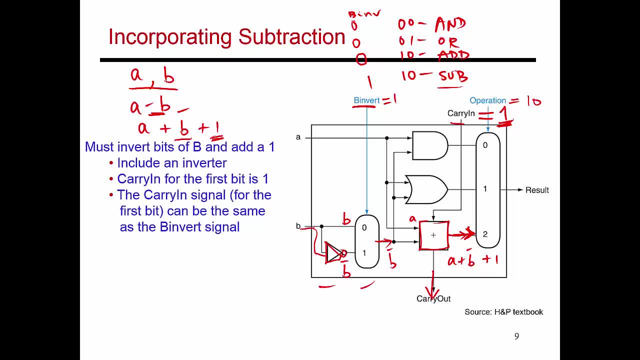 determines exactly what result is going to come out of this ALU, And by setting the signals appropriately, I can pick one of these four possible options. You'll also notice that one simple hack is to connect The carry-in for the first bit to the B invert signal. 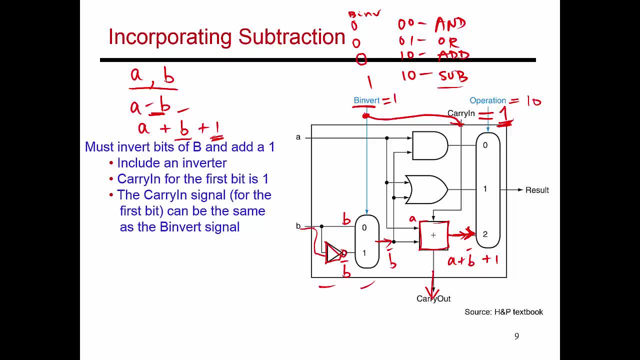 because you'll see that if I'm trying to do a subtraction, I want to set B invert to 1, and I want to set carry-in equals to 1.. And in all other cases I want to set B invert to 0. 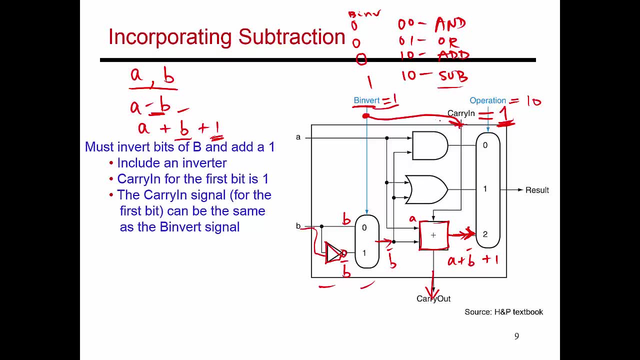 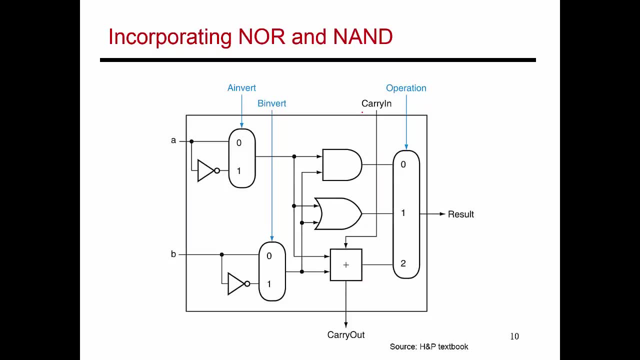 and carry-in to 0 as well. So essentially this carry-in can be connected to the B invert signal. Now let's also see how we can use the same unit to perform NOR and NAND as well. So in the previous slide I had circuit. 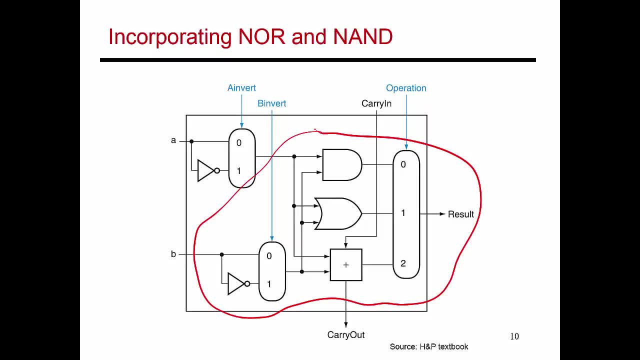 that kind of corresponds to all of this stuff here. What I've done is I've realized that, hey, adding an inverter and a multiplexer is a great way to propagate either B or B bar through the rest of the circuit. I can do the same thing for A. So now I've 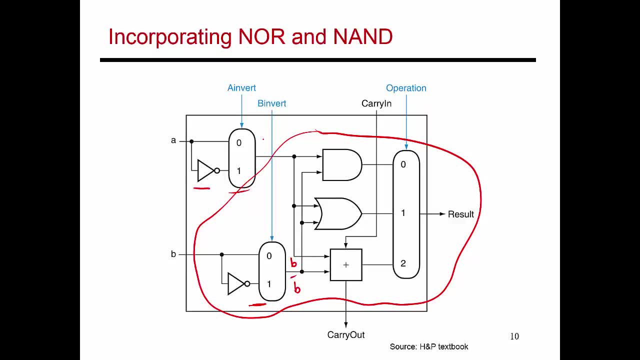 added an inverter and a multiplexer for A as well, So I can either have A propagate through the circuit or I can have A bar propagate through the circuit, depending on the value that I set for A invert. So for both this AND gate and this OR gate its inputs. 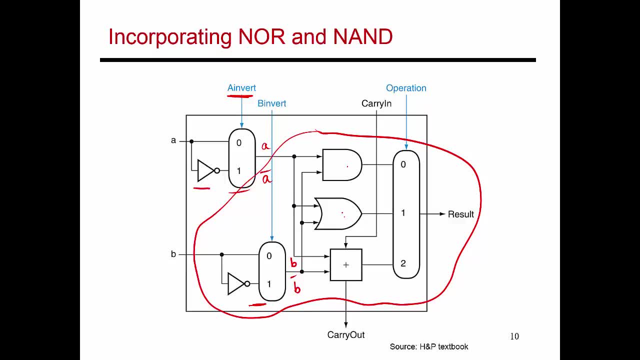 need not be just A and B. The inputs can also be A bar and B bar. So this adder, for example, is capable of doing A bar dot B bar which with De Morgan's laws is nothing but A plus B, the whole bar, which.